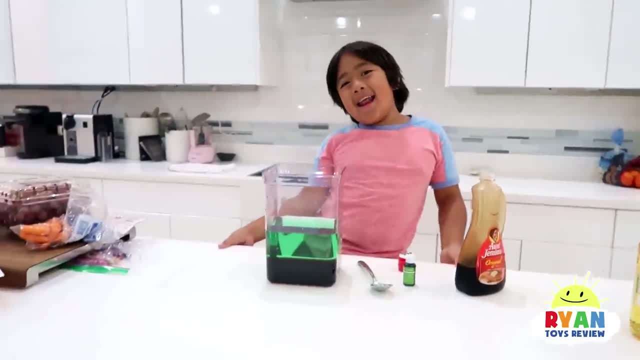 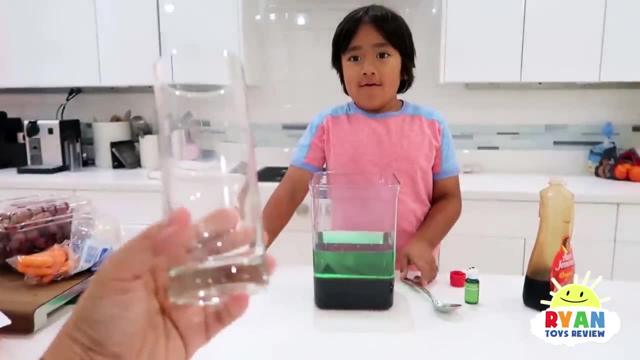 Just a little bit more. It's done, Yeah, so you guys don't have to do it in a giant container. We're doing it in a giant container to show you guys, But you can also just do it in a glass or any small container, right? 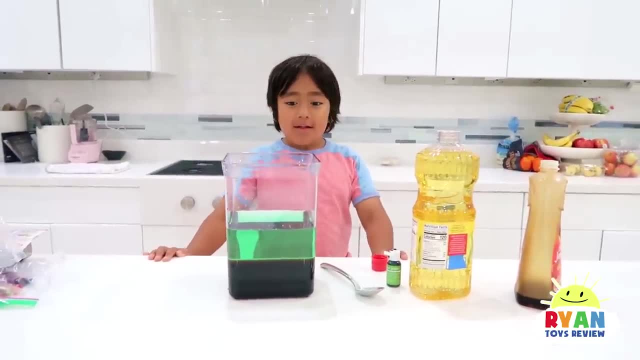 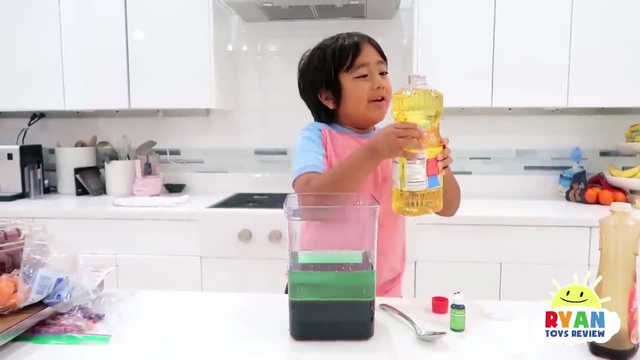 Yeah, We're going to put in corn oil. Yeah, or any cooking oil will do. What do you guys think? Will corn oil mix with water or go to the bottom of the water? I think it's going to float. It's going to float so it's less dense. Let's see what happens. 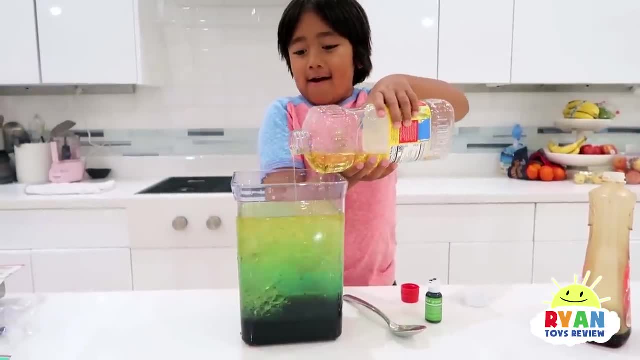 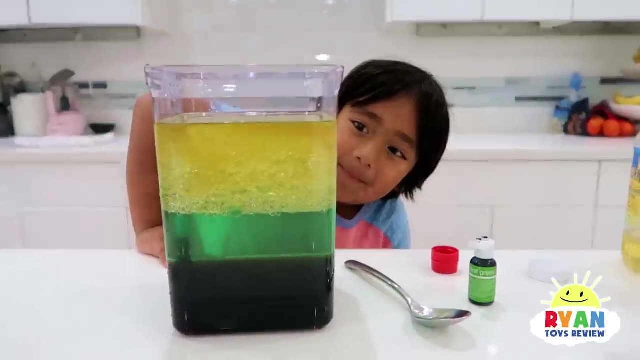 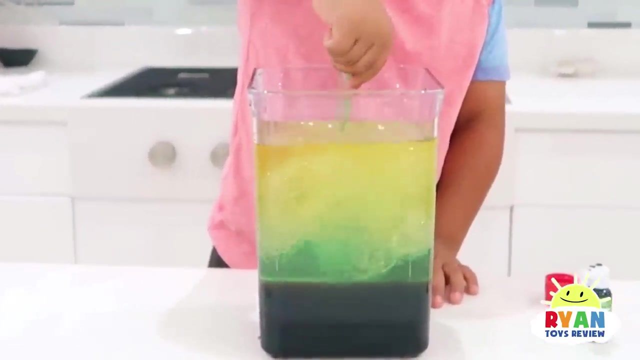 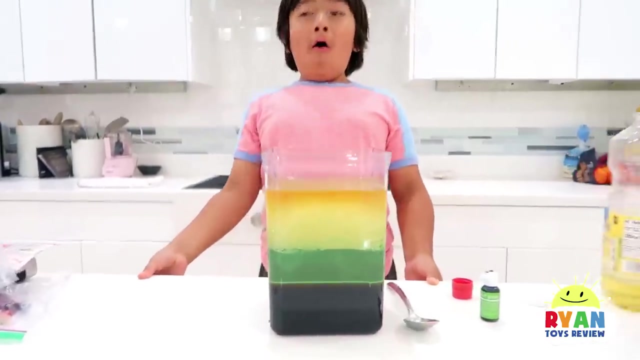 All right, Whoa. So what happened? It floats. Yeah, so that means oil is less dense than water, right, Let's see? Even if you try to mix it, Whoa, it still separated out. Yeah, so now we're going to wait 10 minutes for all the layers to separate. 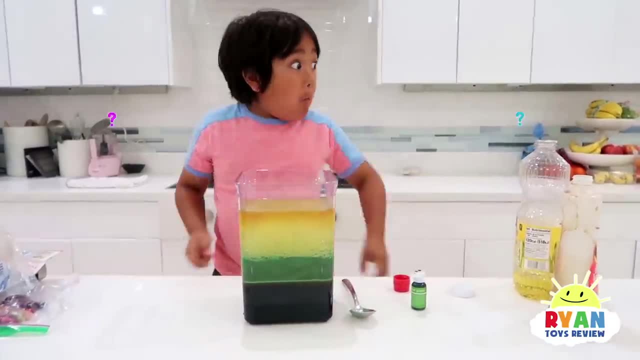 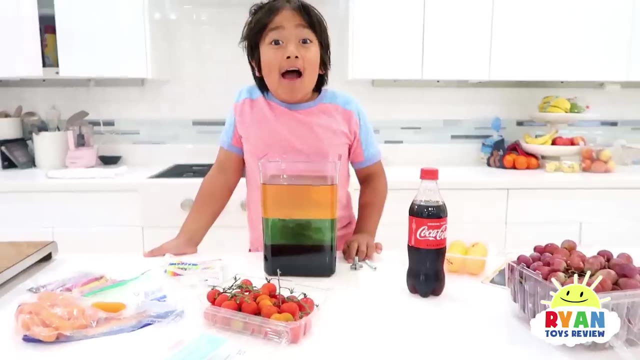 And then we're going to look around the house to see what things will float on which layer. Okay, We'll be back in 10 minutes, 10 minutes later. Okay, guys, It's been 10 minutes now. And now we're going to see which items sink or float. 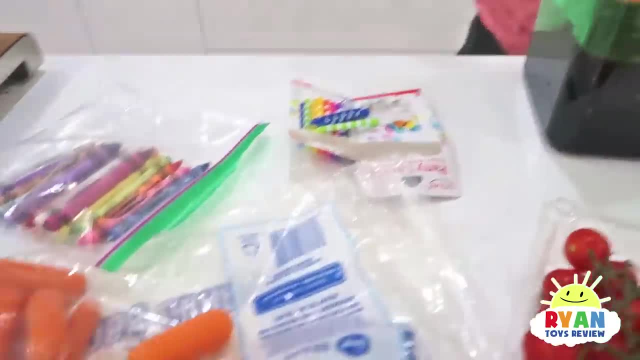 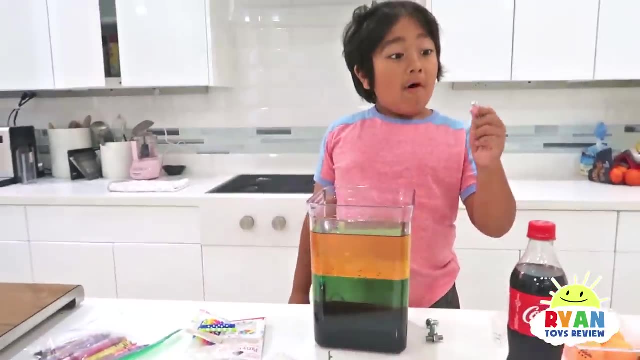 That's right. So we just went around the house and gathered some items And we're going to test each object to see where does it place in the density column. I think this is going to go all the way down. So first, Ryan has a screw. 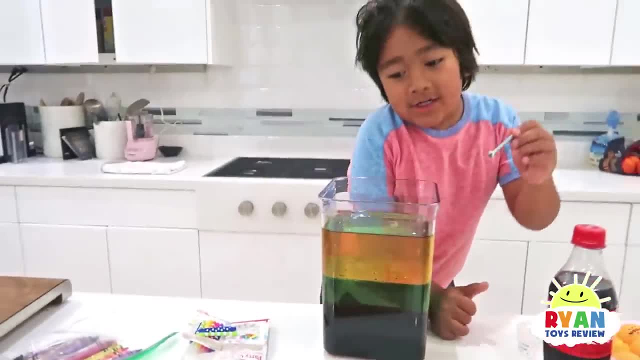 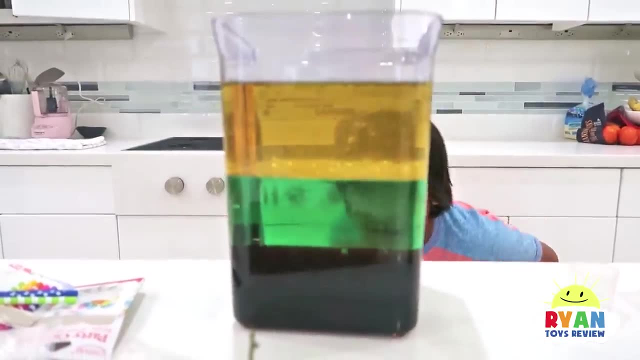 Right. So Ryan thinks it's going to sink all the way down. We can try all the screws: Three, two, one, Whoa. So what happened? What are they? It went all the way down. That's why we didn't see it, because the bottom layer is too dark. 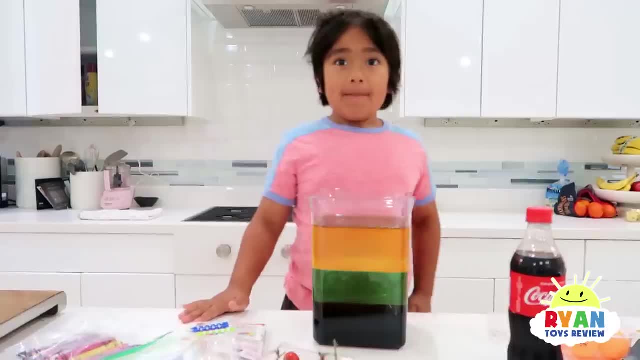 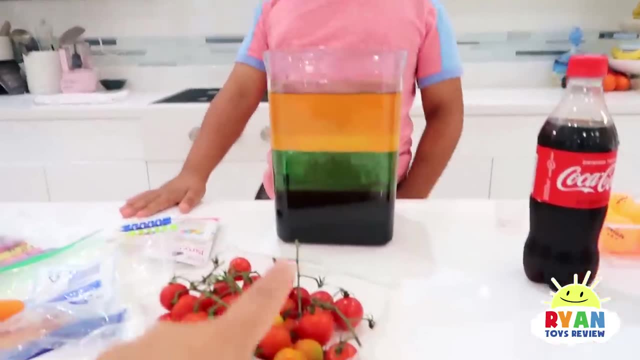 So that means it's very, very dense. Is the screw more dense or less dense than water? More More, Way, more dense. That's right. It sank all the way down. Okay, What object do you want to test next? 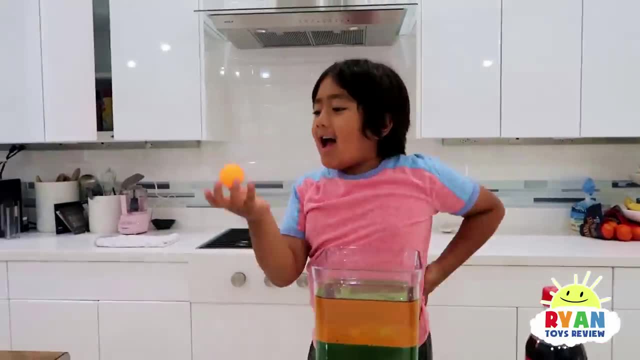 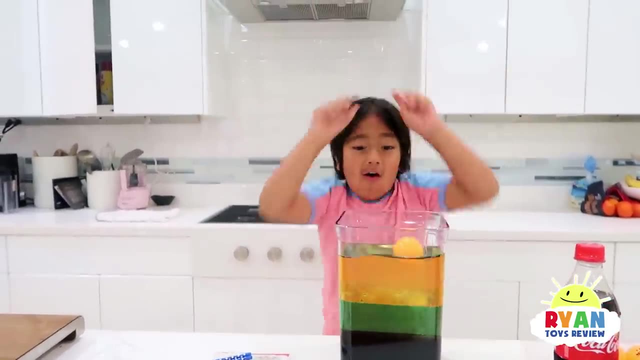 Let's try these Ping pong. Okay, What do you think? before you put it in, Maybe like under the corn, Under the oil? Yeah, Okay, Let's see. So what happened? Whoa, It floated, It floated. 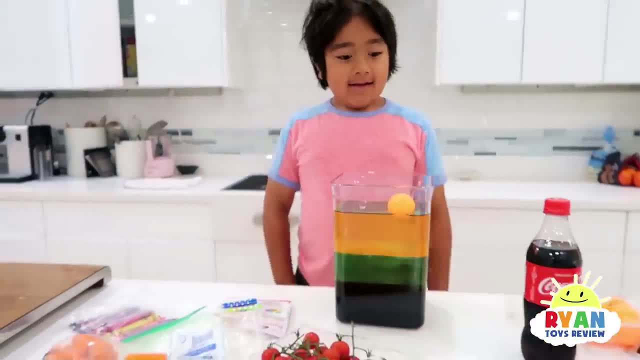 So the ping pong ball is actually less dense than all of them. Right, Try to push it down, Let's see what happens. Uh, Does it go down? No, No, It just keeps going back up. Let's try birthday candles. 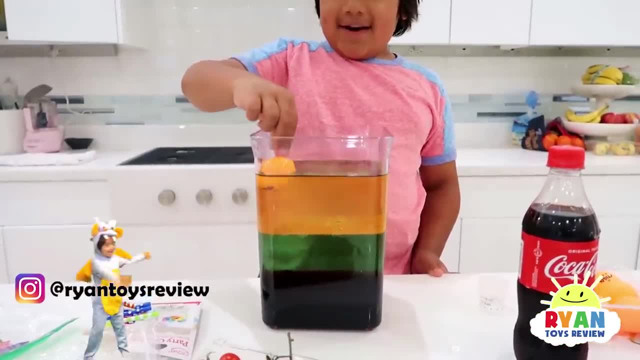 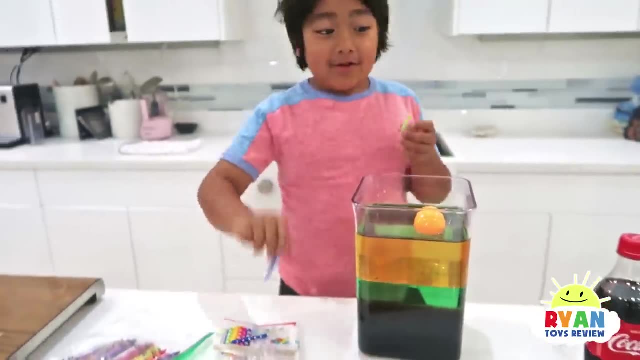 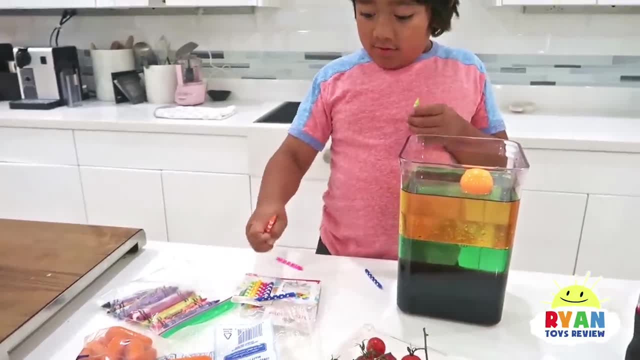 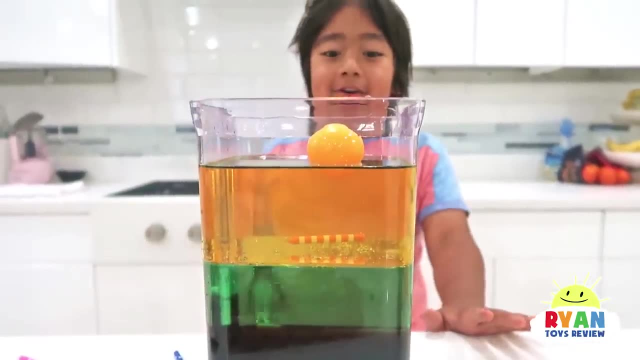 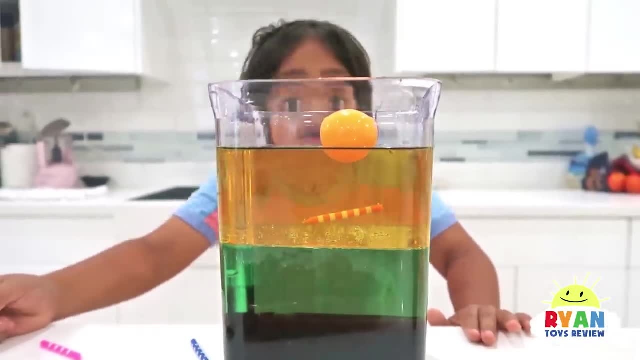 Let's see if the colors and sizes make a difference. Okay, It went right under the oil, That's right. So it went under the oil, but it's on top of the water, Right? Yeah, Uh, oh, It's floating back up. 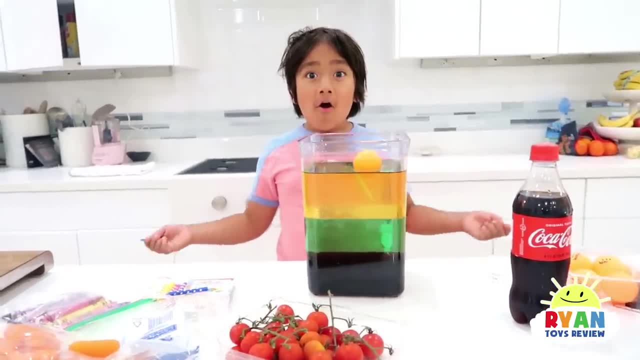 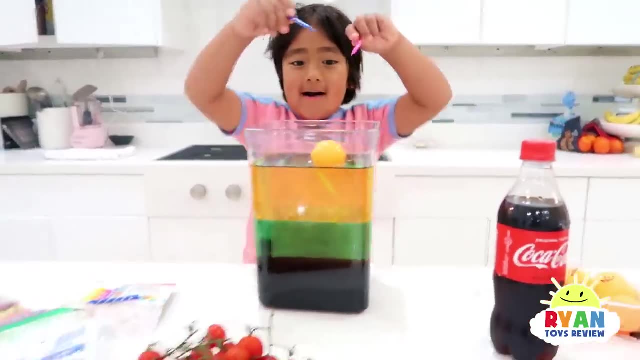 Uh huh, Let's get it. So does this mean the candle is more dense or less dense than water? Less dense, That's right, because the water is the green, right? Okay, what other objects do you want to try? You want to keep trying the candles. 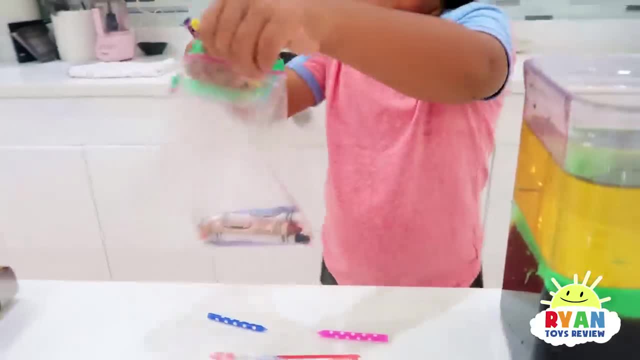 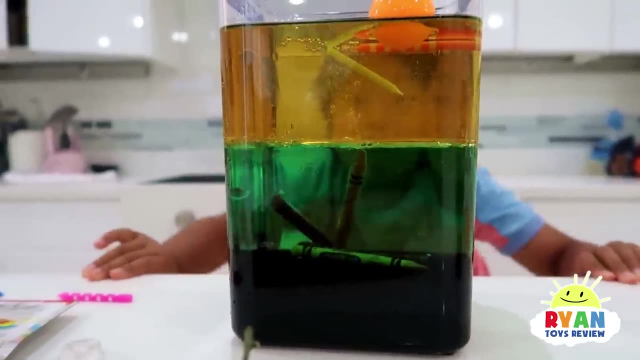 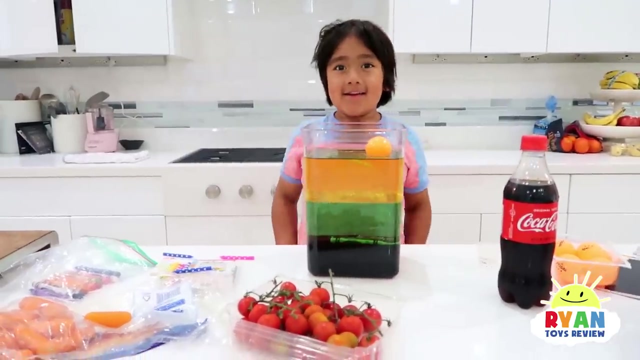 I want to try crayons. Ooh, that's a good one. Let's try four crayons. You have space. Let's see What. Whoa. So what happens? It's way more dense than everything. It's way more dense than water. 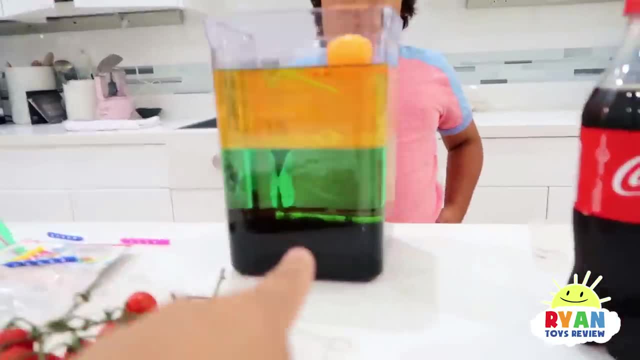 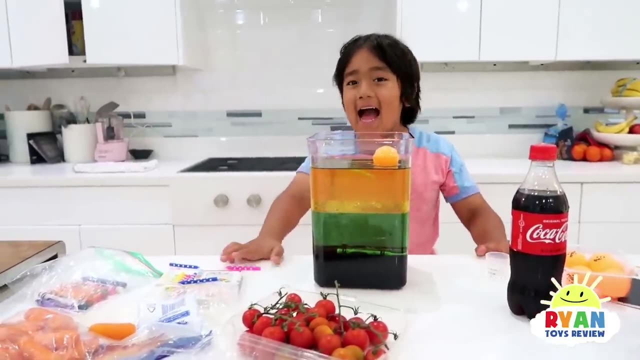 And way more dense than oil. That's right, but it floats on top of the syrup, Do you see? Oh yeah, it's not all the way down, So that means it's less dense than the syrup. Yeah, Okay, what else do you want to try? 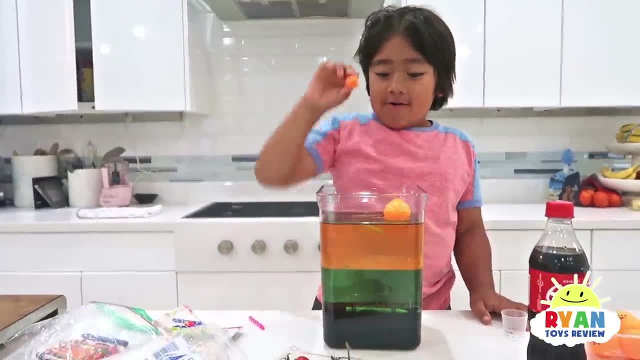 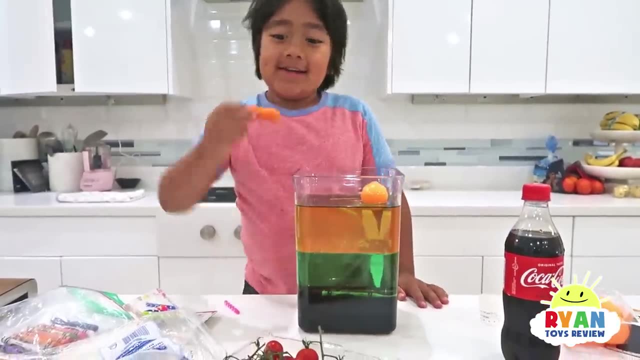 That's fun. This one's big. What do you think? Before we put it in, where do you think it's gonna lay? in the column Right on top of the water? So it's less dense than water, Maybe. Okay, let's see. 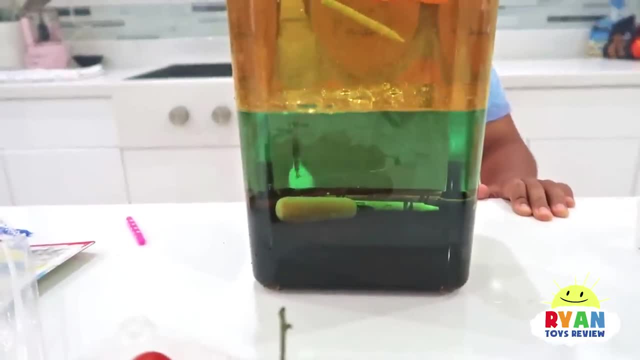 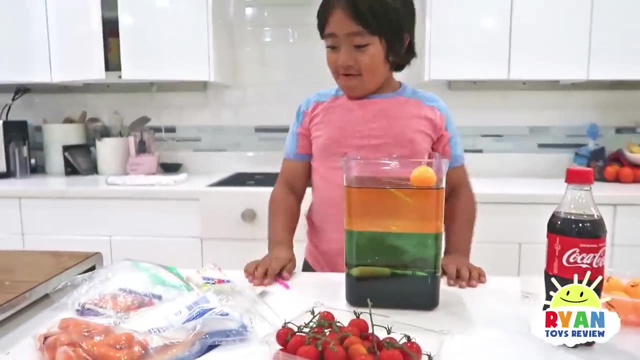 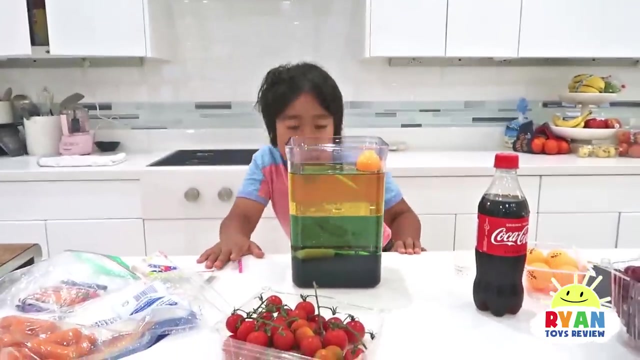 Yeah, Or it just goes all the way down, Hi Ryan, Hi, hi Ryan, Whoa, Whoa. So it is more dense or less dense than water. It is more dense, That's right, And less dense than syrup. 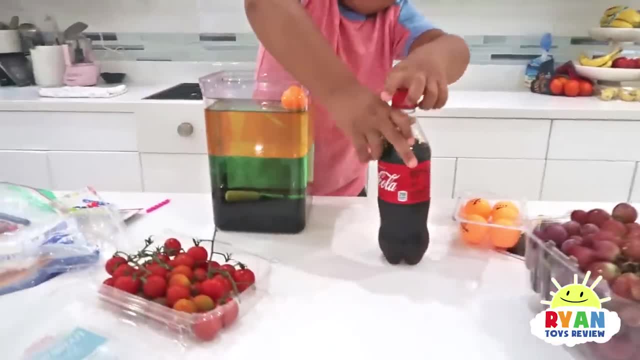 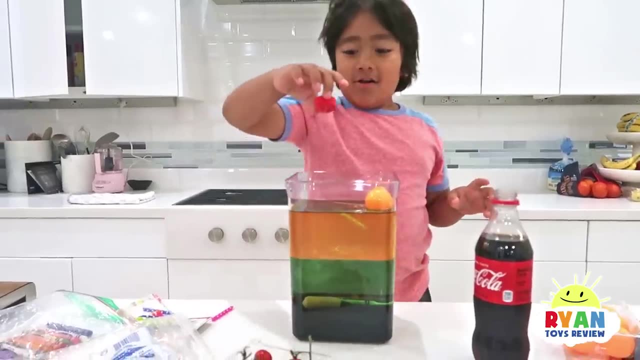 That's right, good job. Okay, what else do you want to try? I'm gonna try the cap. Okay, Where do you think the cap goes? Probably on the water, In the middle of the water. It's gonna float, it's gonna float. 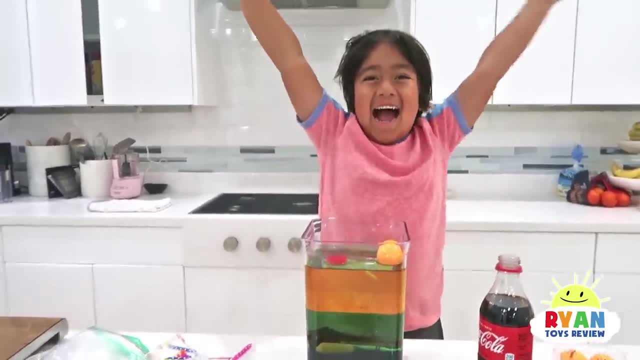 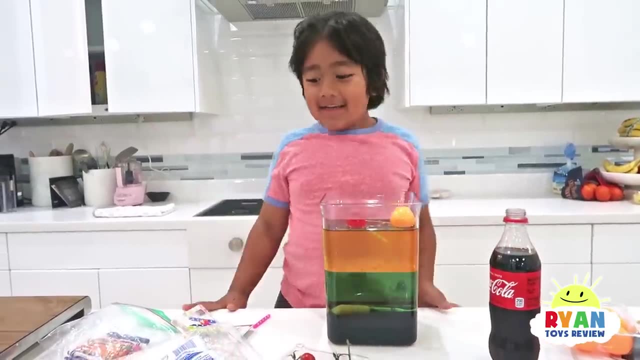 On the very top. Yeah, Okay, let's see. Yeah, Good. So what does that mean for the cap? It's less density than everything. That's right, good job. Okay, so we have some other food here. we're gonna try. 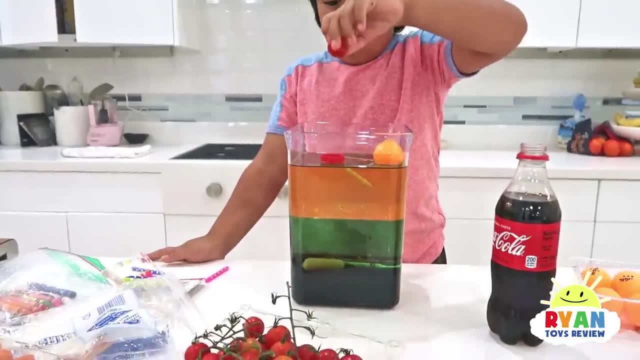 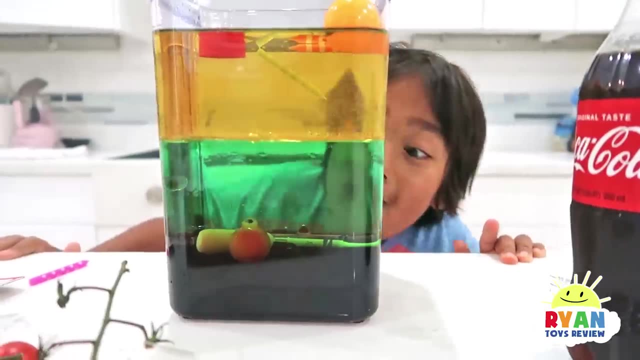 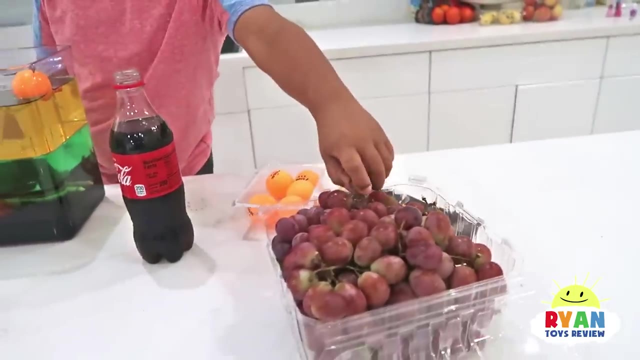 That's kind of fun, Cherries. Yeah, Oh boy. Oh, it's less than syrup, That's right, less dense than syrup. Okay, we also have grapes here. Let's see what matters. Oh, I'm gonna get the big one. 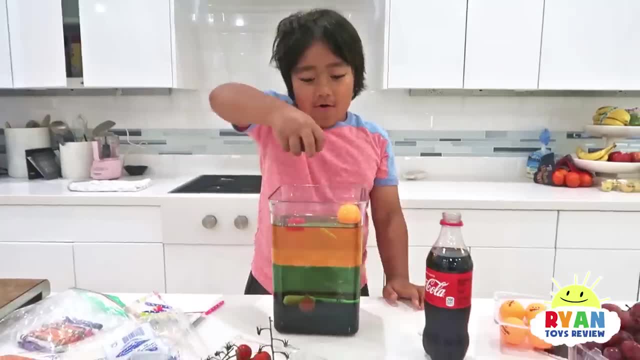 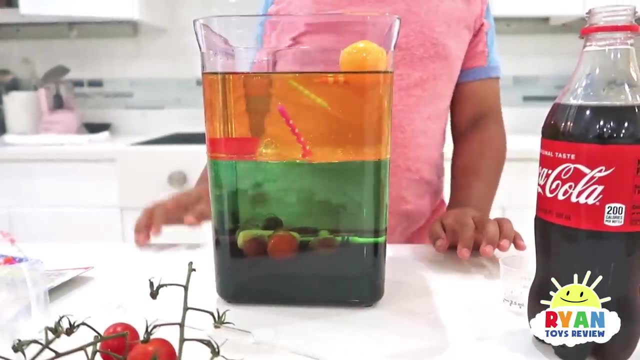 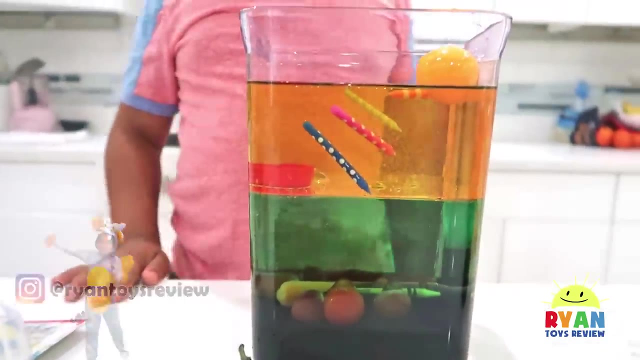 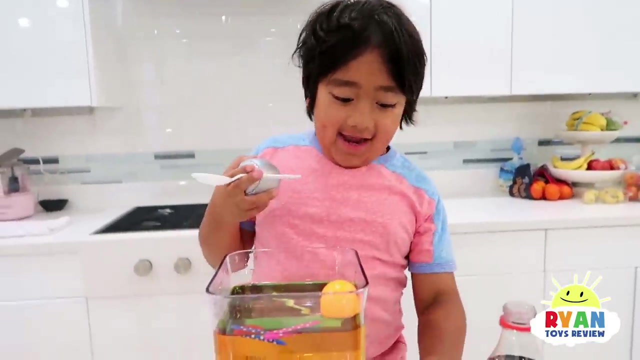 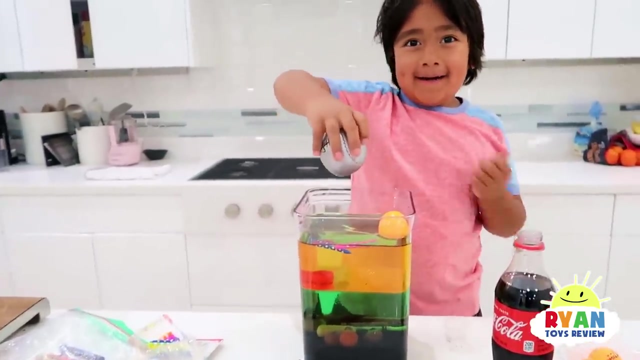 Okay, Ryan's gonna see if the big one makes through difference. so it's more dense than water but less dense than the syrup. well, that's kind of cool. yeah, I just came back for a few more items, so I have this a ball, okay. so what do you wanna try? first wait before you put it in. 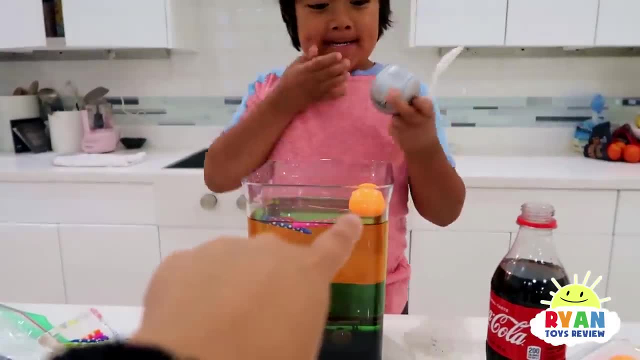 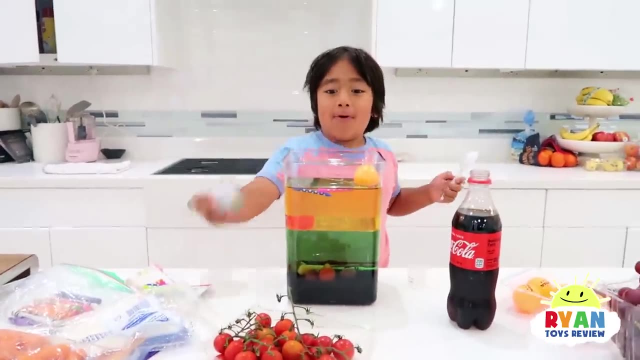 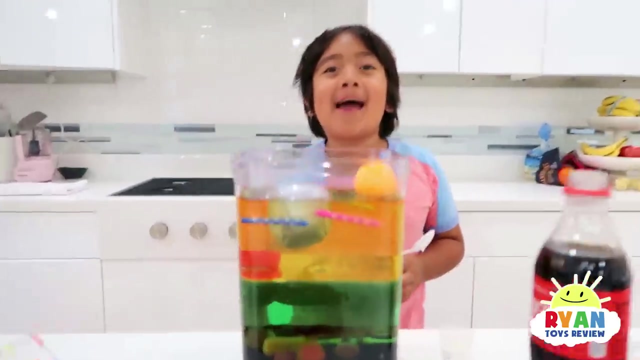 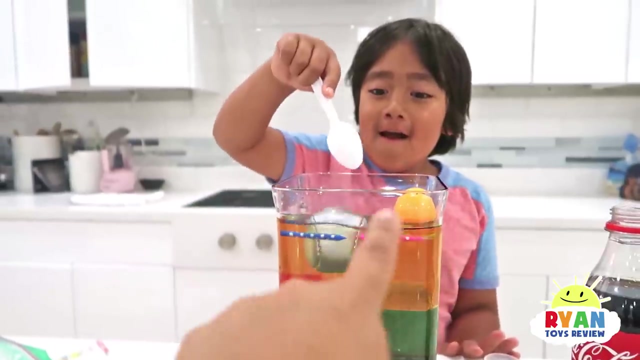 so that's a ball and that's also a ball. so the ping-pong ball floats. but what do you think about the juggling ball? okay, let's see if mine's right. no, I did it, but it did sink a little bit, so maybe the density of this juggling ball is more. 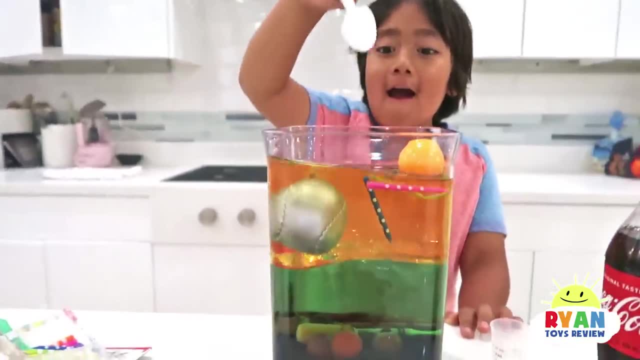 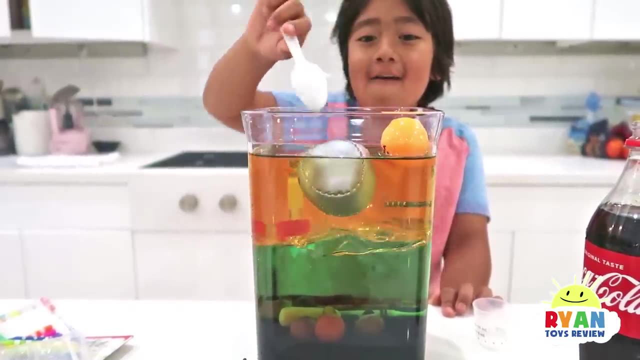 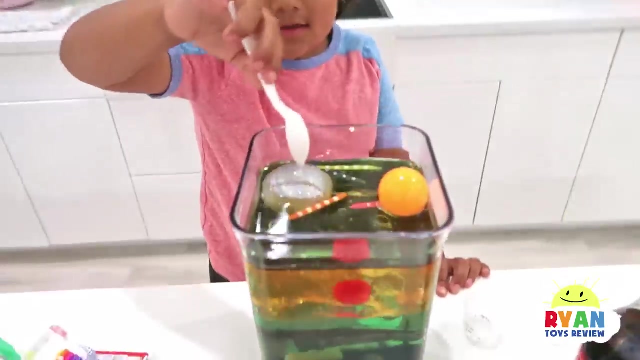 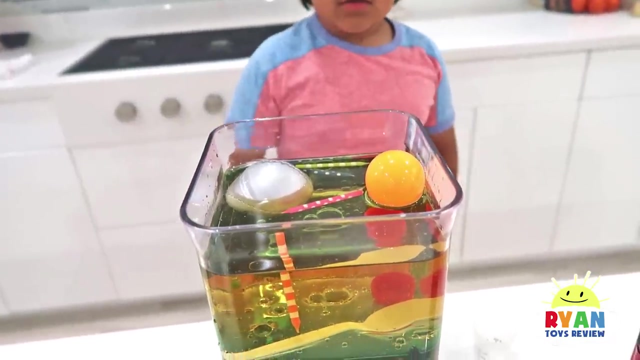 than the ping-pong ball, but it's still less than water, right? definitely. so it's a juggling ball. more dense or less dense than water? that's less than. yeah, it's actually less dense. is it less dense than this? well, it goes down a little bit, so that means it is less dense. oh then, same sense, yeah, wait. 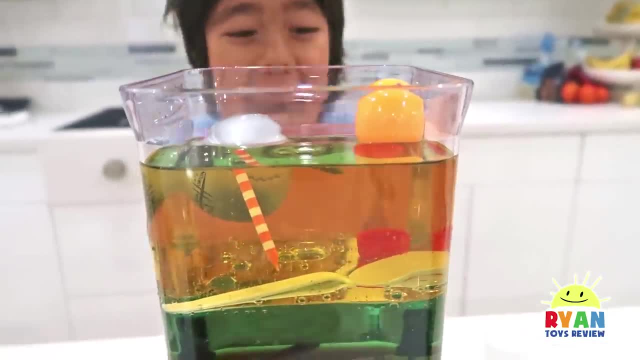 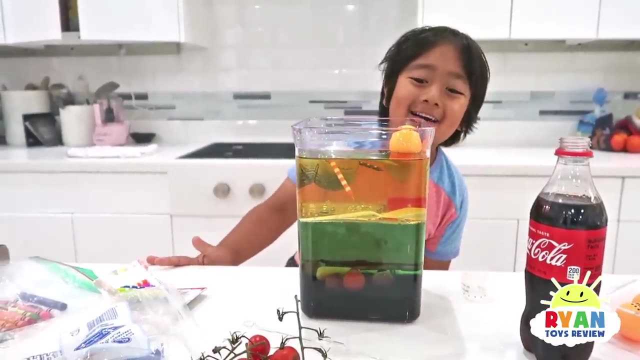 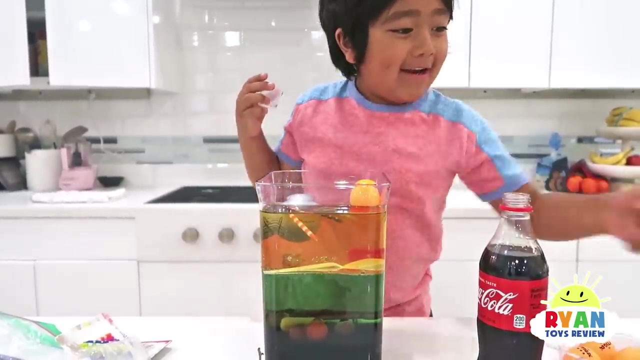 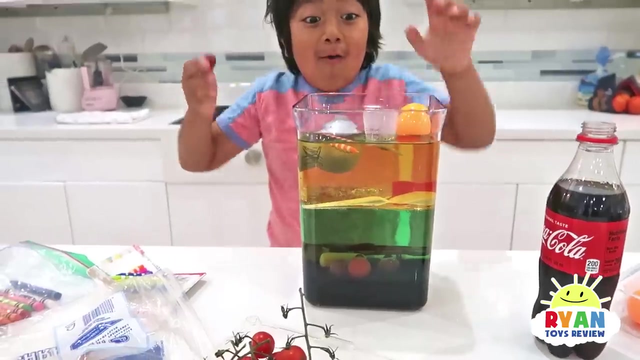 well, look at the spoon. it just floats on top. oh yeah, just like the cap. wait, how the cap? that all because you flipped it upside down. oh so let's try super small cup. yeah, the medicine cup we use. what do you think before you put it in? oh, I think it's going to go to water. okay, let's see what. 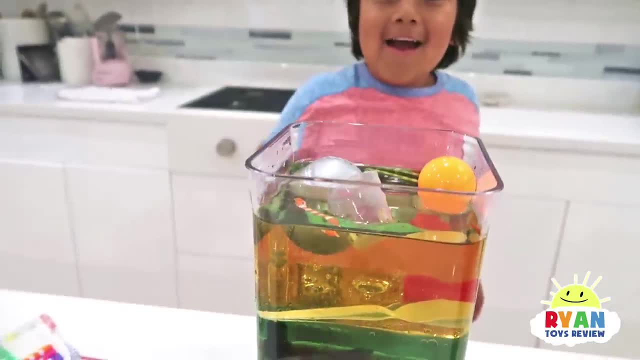 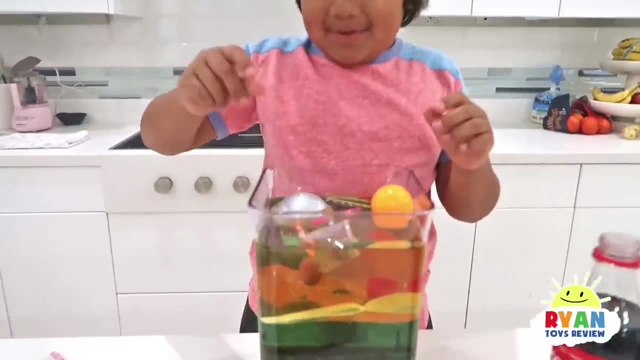 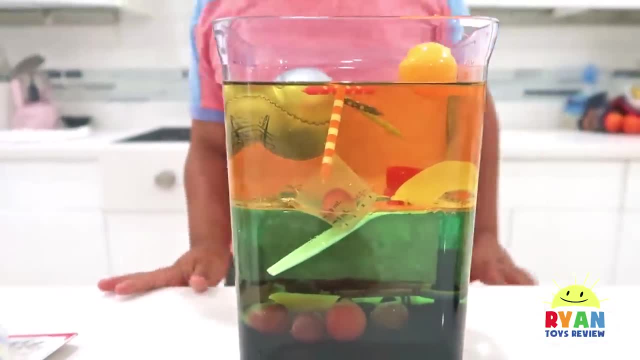 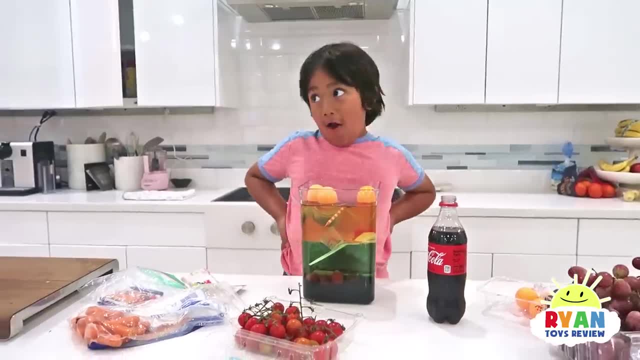 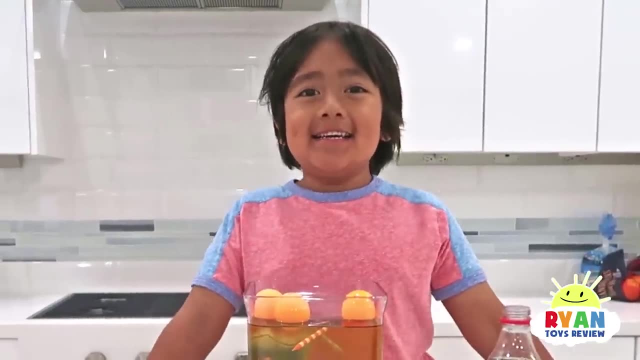 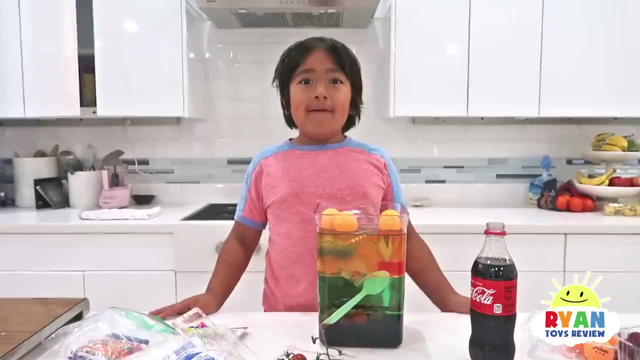 Woo-hoo. So before we go, I have a question to ask you: What is it? Why do things sink or float? Because they have density, That's right, And if the density is less than water, it will. It will float. 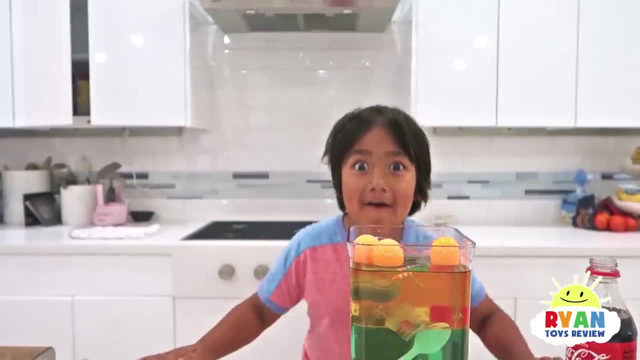 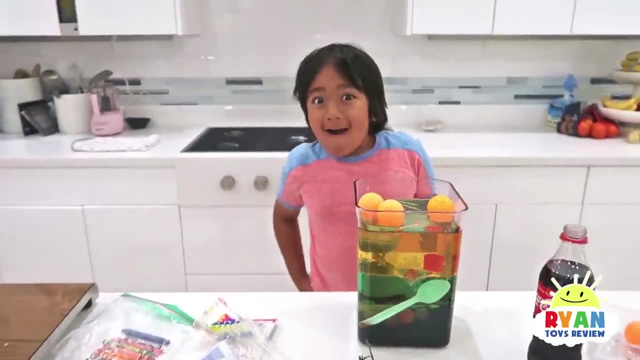 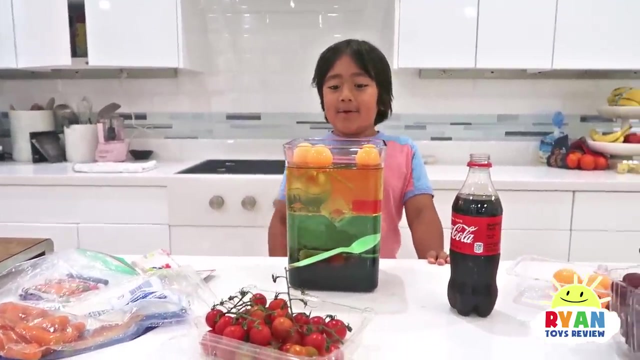 If the density is greater than water, it will sink. Good job. And you can tell that different liquids also have different density, right Yeah? So out of those three liquids, which one is the least dense? The least one is oil. 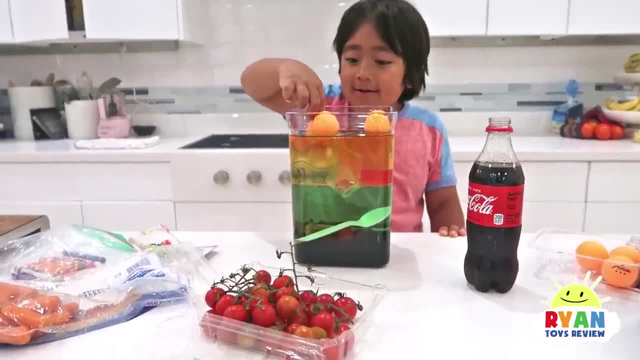 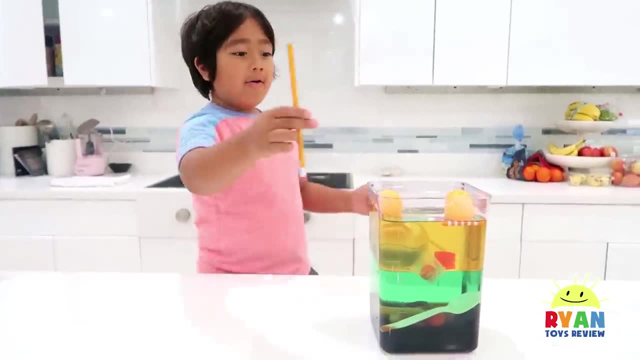 That's right. Wait, it's going down. it's going down. What is going down? The ball? He's weighing everything down. Okay, guys, and last we're gonna try pencil. Let's see if it float or sinks. 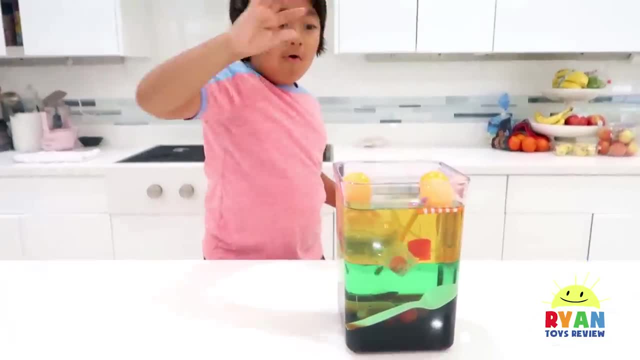 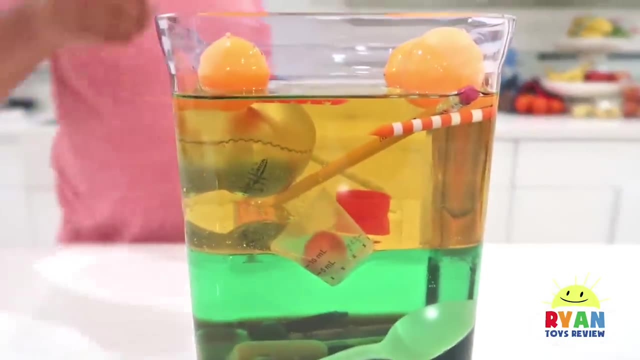 I think it's going to float. It's a little, is it more than water? Yeah, it's floating on top of water. Ooh, And then a pencil eraser here, Oh, Oh, Oh. I want to set the camera. 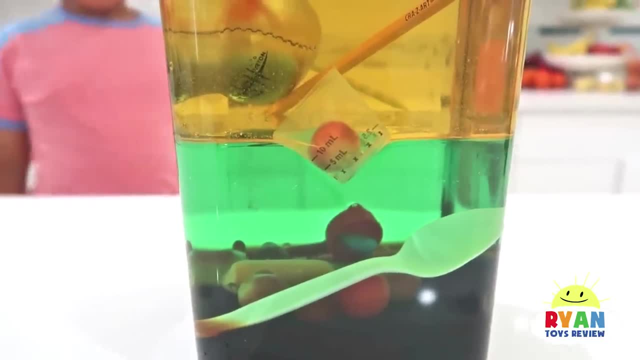 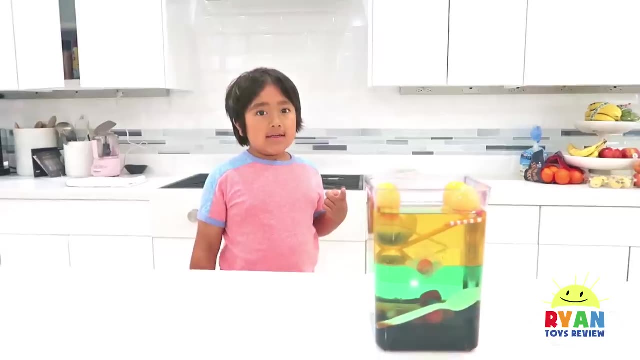 Oh wait, it's sinking, Oh Whoa. So what does that tell you? A pencil is more or less dense than water. Oh, it's technically less Good. it's because it's on top of water, right?